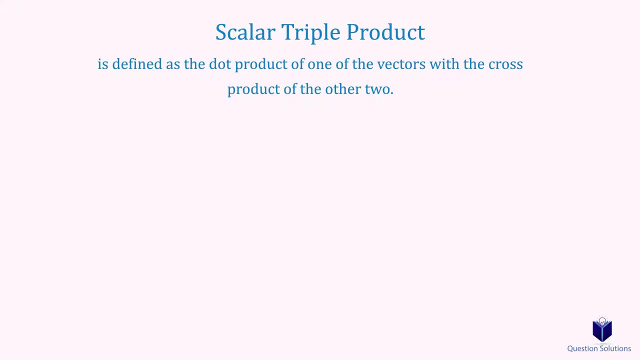 Let's go through how we can solve a triple scalar product In this video. I'm not going to go into the math behind this, but rather how we can solve it fast and simple to get a solution. The process to solve this involves multiplication, addition and remembering a few steps. 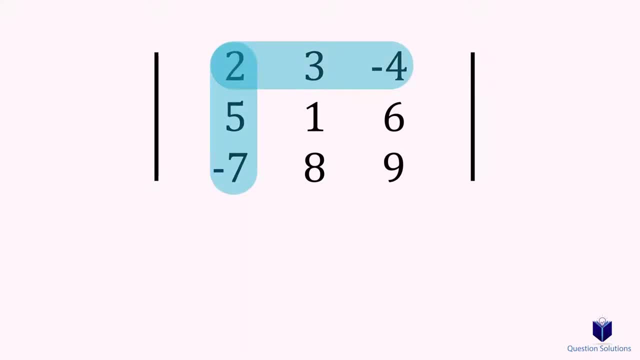 The first step is to cover the top row and the very leftmost column. Next, we will write down the intersecting number. In this case, it's 2.. You will notice that, since we covered the row and column, it leaves a box of numbers available, which are 1,, 6,, 8, and 9.. 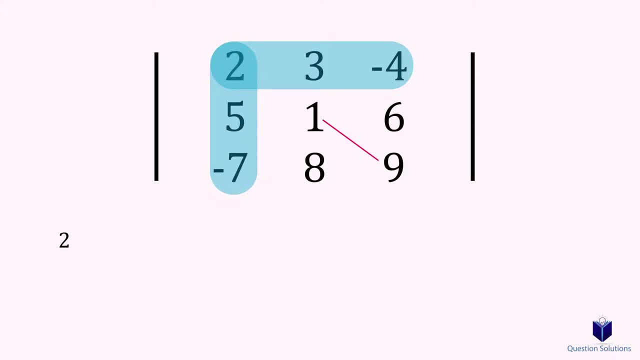 We will first multiply across from top left to bottom right. That would be 1 multiplied by 9.. The next multiplication will be subtracted from this value, so we will write a subtraction sign. Next multiplication is top right multiplied by bottom left corner, which would be 6 by 8.. We 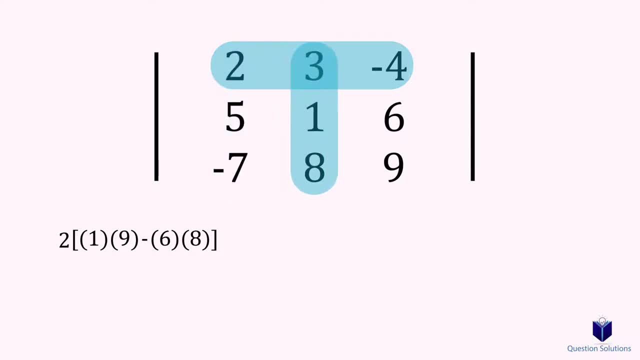 will now cover the top row and the middle column. When we do this, the intersecting number becomes 3.. So we will write down the intersecting number. In this case it's 2.. You will notice that, since we covered the top row and column, it leaves a box of numbers available, which are 1,, 6,, 8, and 9.. We will 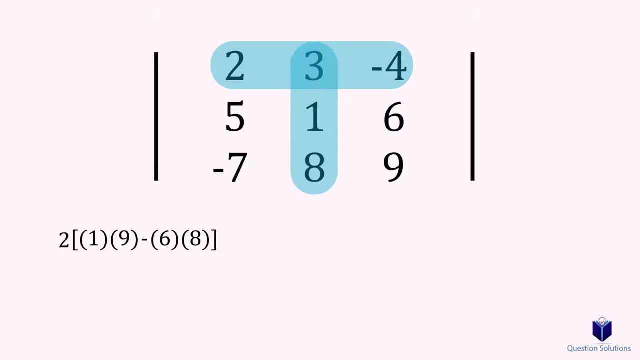 also write down the intersecting number. Something to remember which is very important is that every time we switch the column we cover, we have to change the signs. Since the beginning was positive, the next is negative, so our intersecting number becomes. 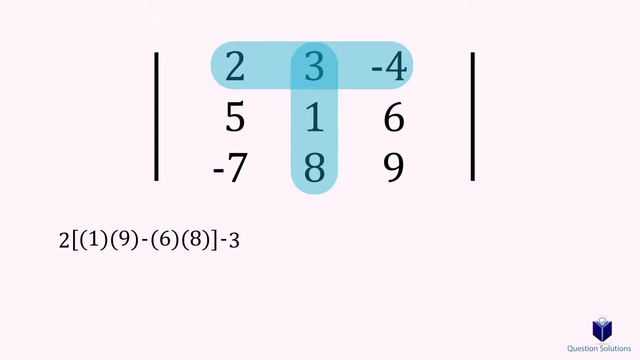 negative 3.. As before, we are left with four numbers that we will cross. multiply First 5 by 9, and then the value of 6 by negative 7 is subtracted Once again, we will cover the top row. 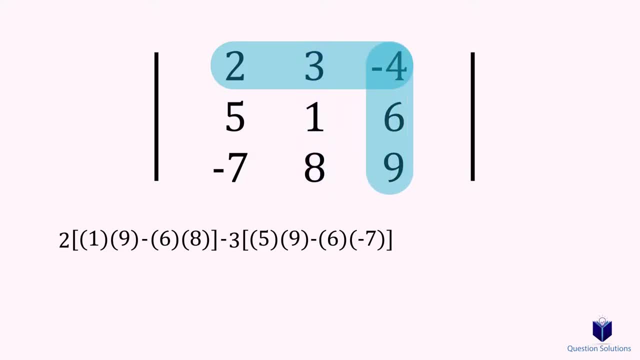 and cover the rightmost column. Now we are back to the positive sign again and the intersecting number becomes negative 4. We will cross, multiply First 5 by 8, and then 1 by negative 7.. Don't. 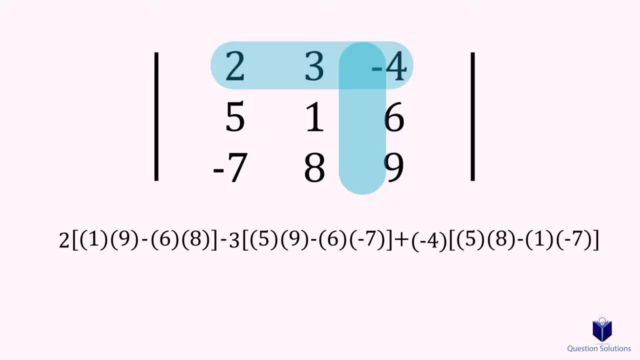 forget to subtract. as before, Every time we switch covering a column, the sign must change, Starting from positive, then negative and then finally back to positive. Now, all that's left is to simplify and solve. Remember that this will give us a scalar value, not a vector value. Let's look at another. 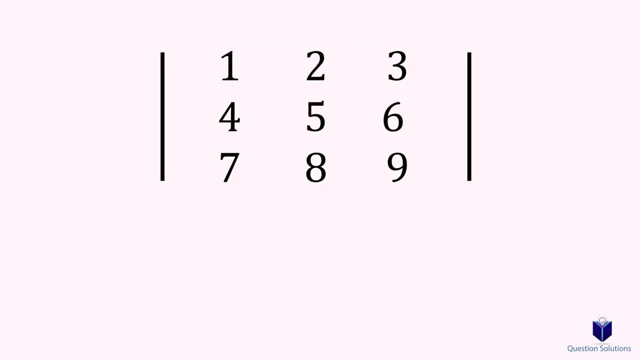 example. Let's look at another example. Let's look at another example. I will go through it faster now As before. cover: the row and column Intersecting number is 1, and we start at a positive sign. Then we cross, multiply the uncovered numbers Top, left to bottom.